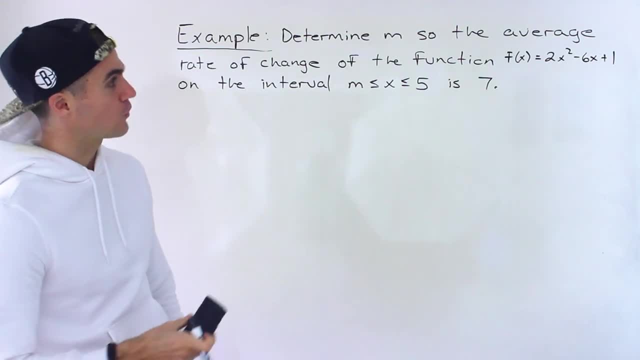 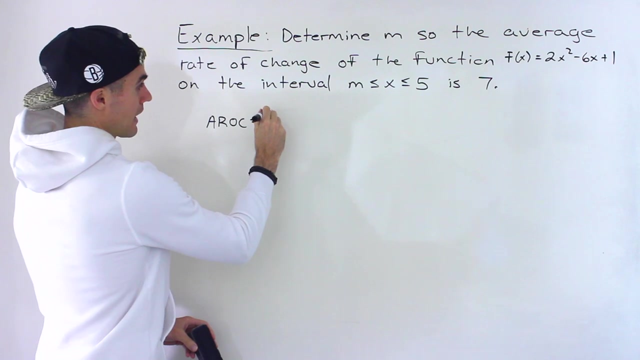 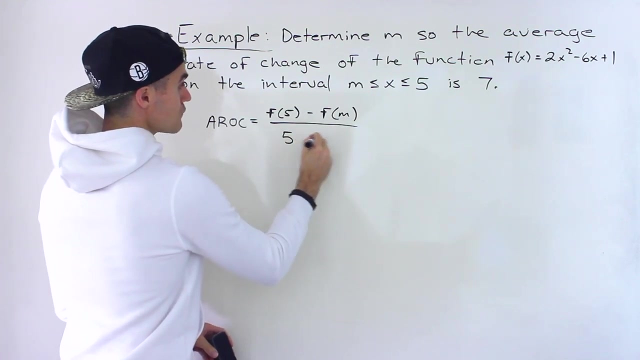 rate of change over this interval is going to be 7 for that function. Now, average rate of change between two values is always what Between these two values. in particular, the average rate of change is going to be f of 5 minus f of m, all over 5 minus m. Right, That's how you set up the 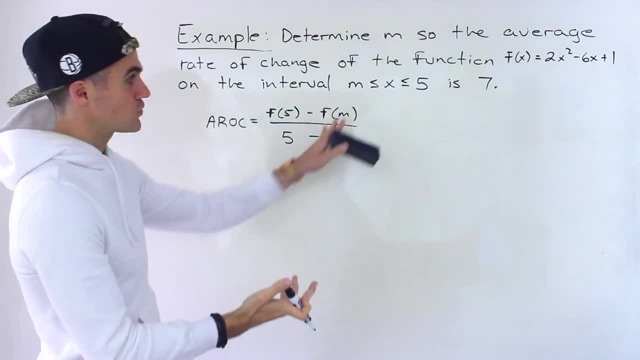 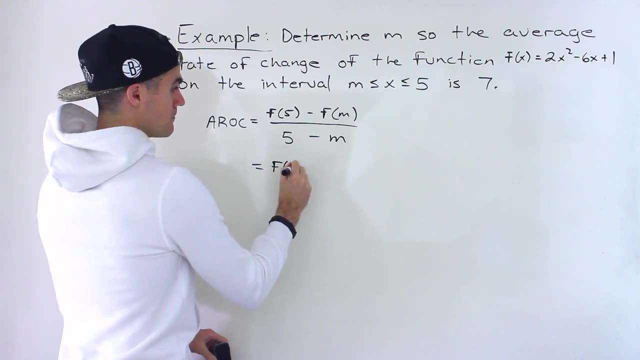 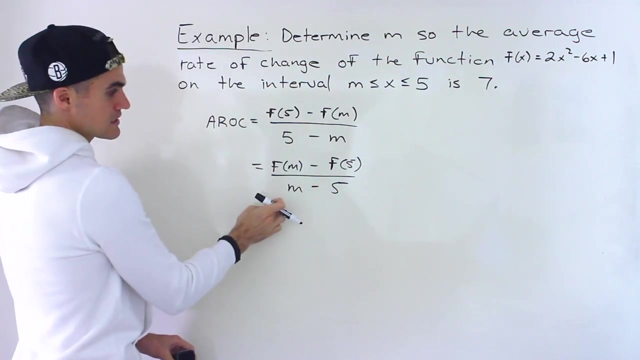 average rate of change. This is the slope of the secant between these two points. Now, it doesn't necessarily have to be in this order. In other way you could do it. you could do f of m minus f of 5, all over m minus 5. right, this and this. 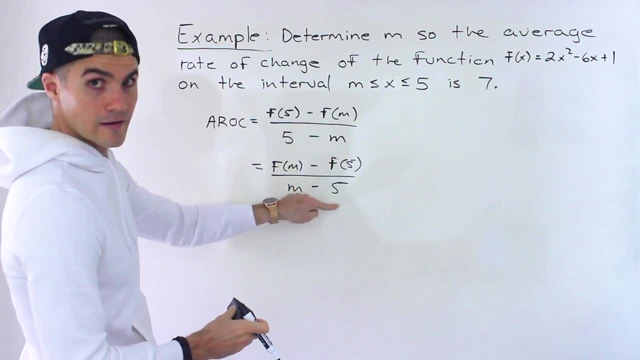 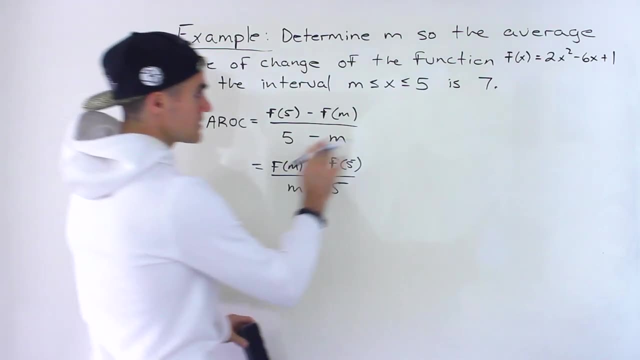 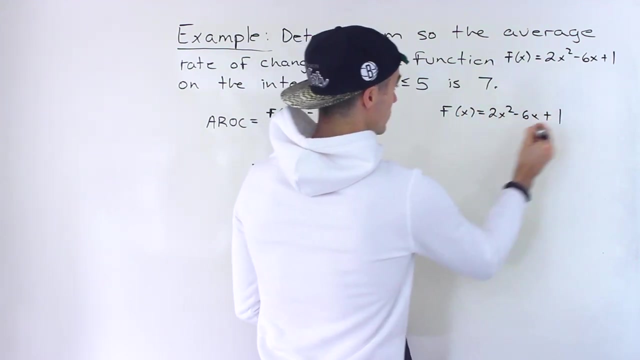 are the exact same thing. as long as these two are lined up, then you can do it in whichever order you want. and I'm actually probably going to work with this order, because notice if on the side, notice how we have f of x equals 2x squared minus 6x plus 1, so if we get an expression for f of 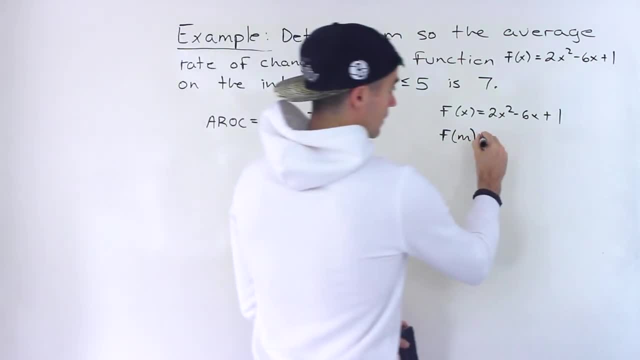 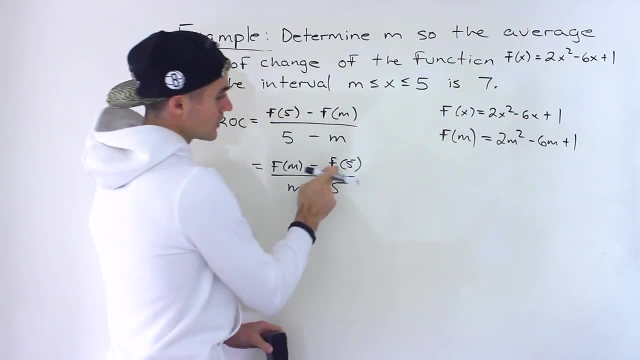 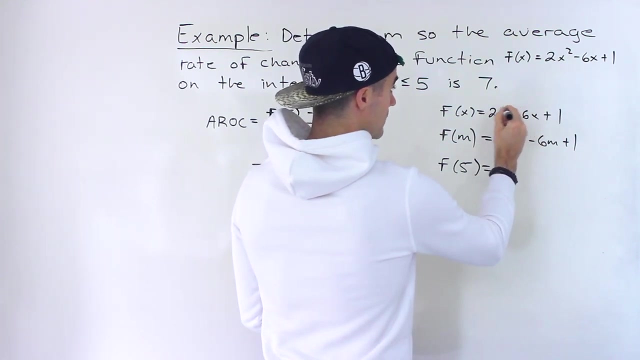 m which we're going to have to plug in here. we would have 2m squared minus 6m plus 1, and then also notice we're going to have to plug in f of 5. so f of 5 would be what? 5 to the power 2 which. 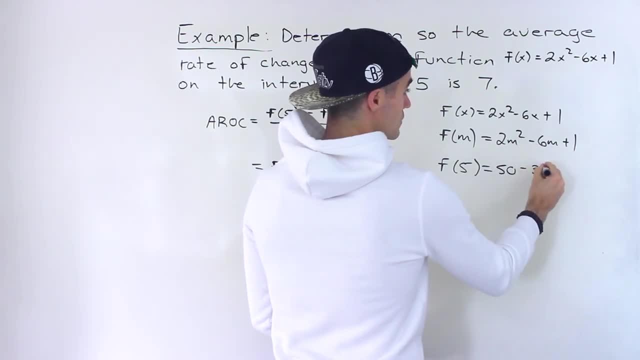 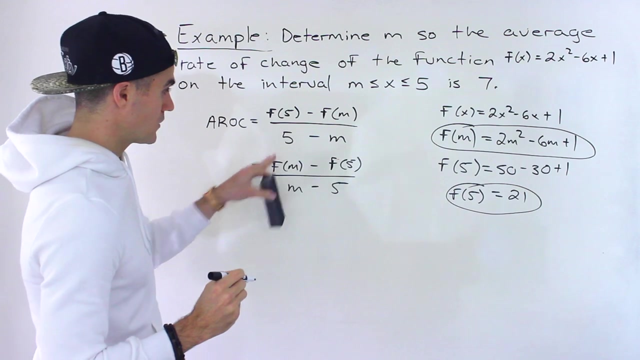 is 25 times 2, is 50 minus 6 times 5, which is 30 plus 1, which gives us 21. that's what f of 5 is. so we have f of 5 equals 21 and f of m is 2m squared minus 6m plus 1. so the reason I prefer to use this one over here: 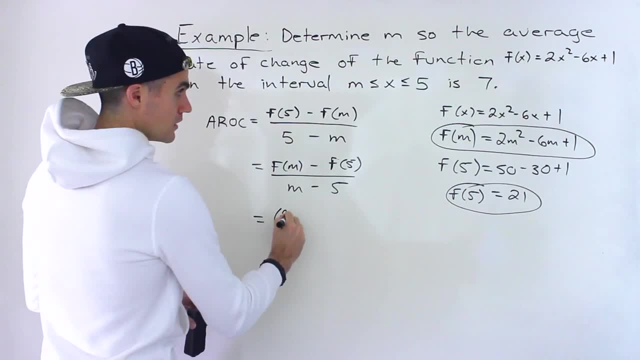 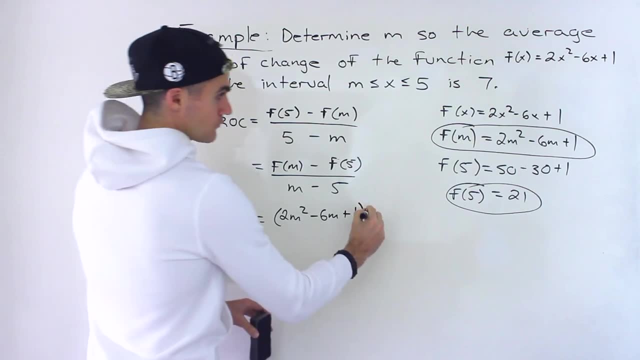 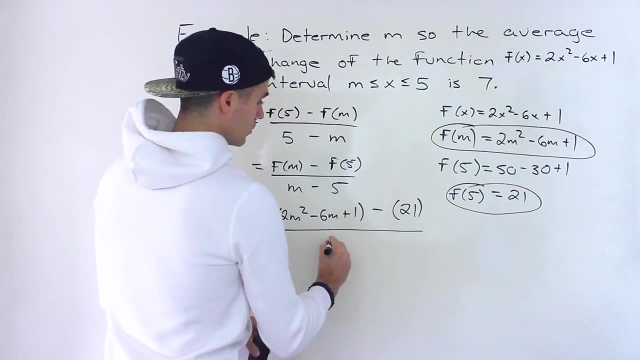 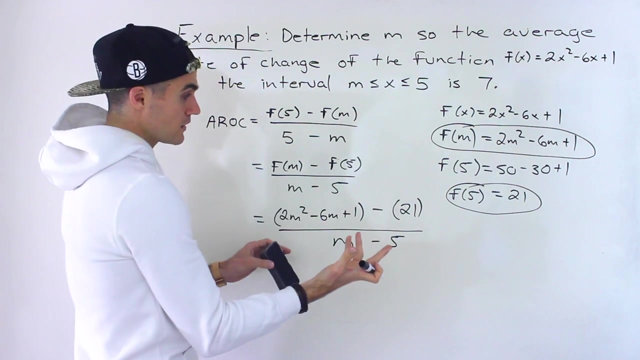 is because when we set it up, that whole expression for f of m, we don't have to worry about distributing a negative. and then this is going to be all over m minus 5, because if we switch these up, which you can do, by the way, you should get the same answer. we could put the 21 minus this. 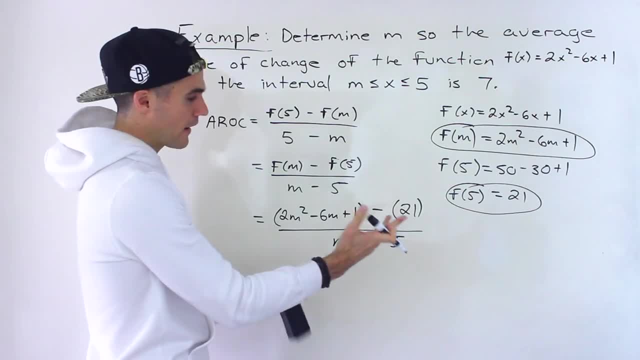 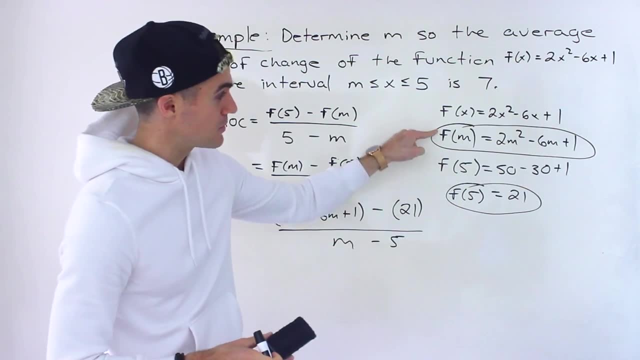 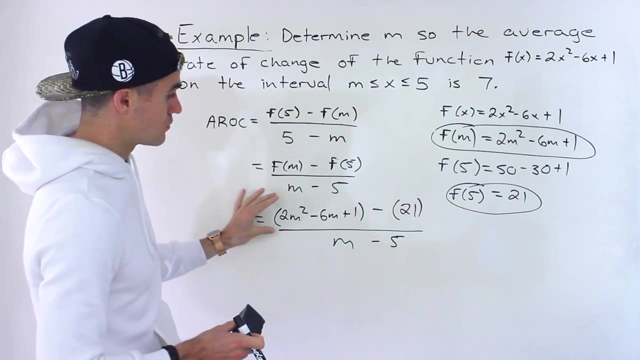 expression here, but then we have to distribute the negative inside the bracket, so there's a little bit more to take into account. so with a question like this, I'd recommend getting these expressions first on the side, so then you can see which order you prefer to put in those expressions. so you 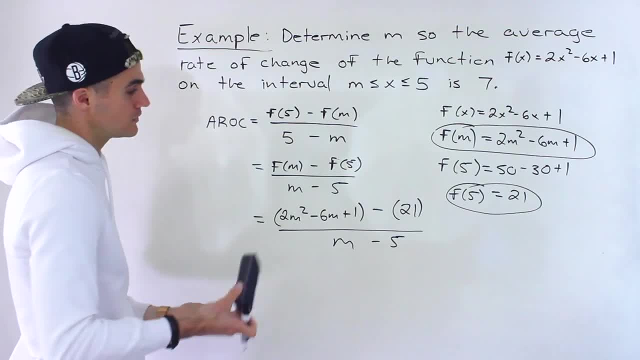 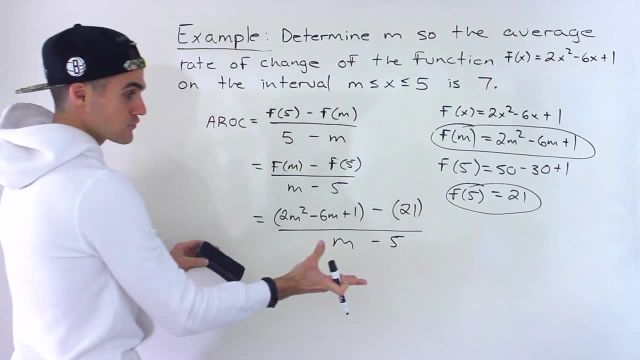 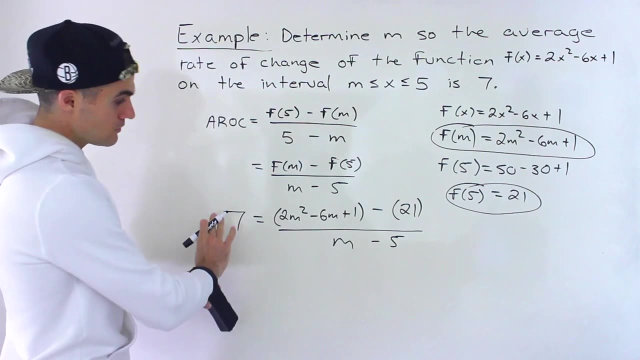 don't have to do as much algebra, but again, it doesn't matter. ultimately you should get the same answer, but personally that's what I do. so this here is the expression for the average rate of change, and we know the average rate of change is equal to 7 in this case. and so now notice we have. 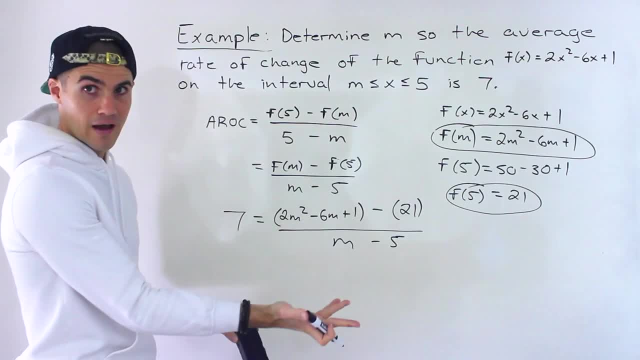 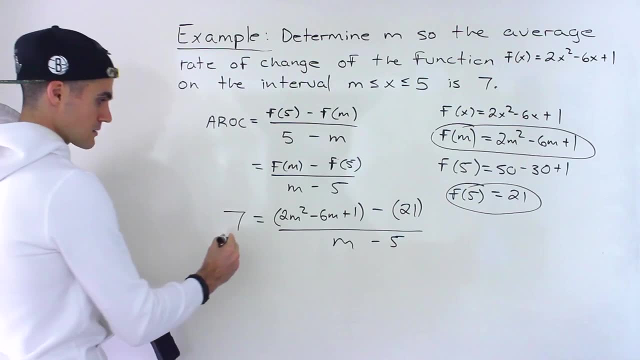 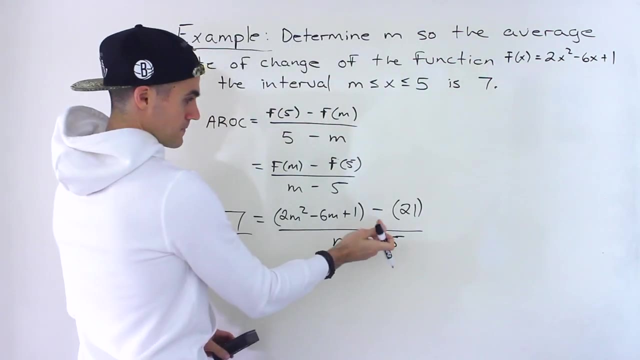 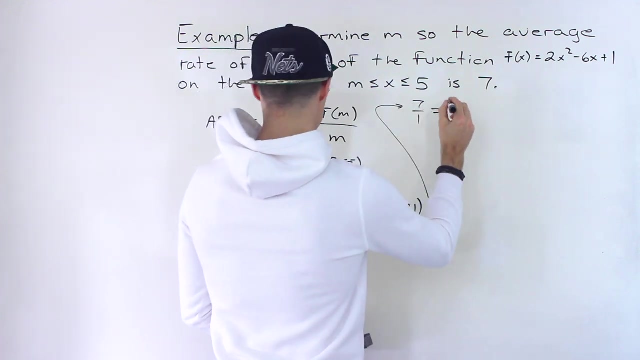 an equation with one variable to solve the m value, which is what we're looking for. so to solve this, what I'm going to do is I'm going to put the 7 over 1. now also notice how we can simplify the numerator here. so we'll have continuing this here: 7 over 1 equals 2m squared. 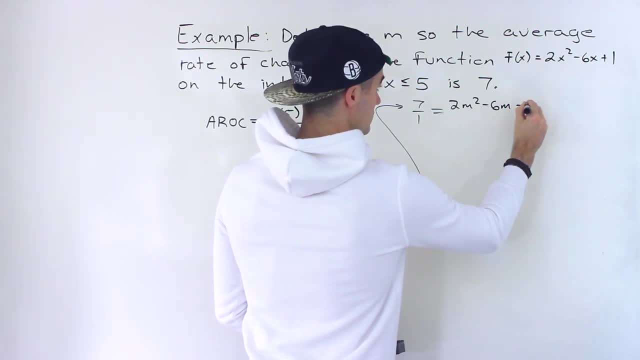 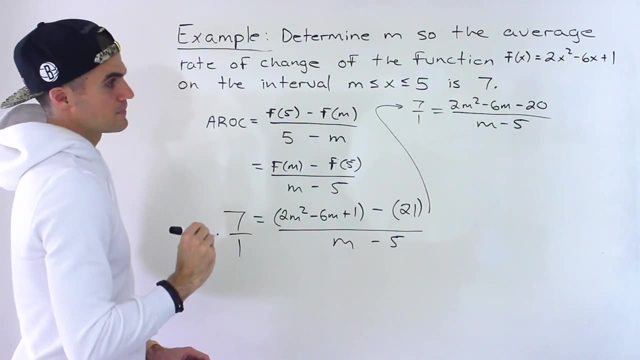 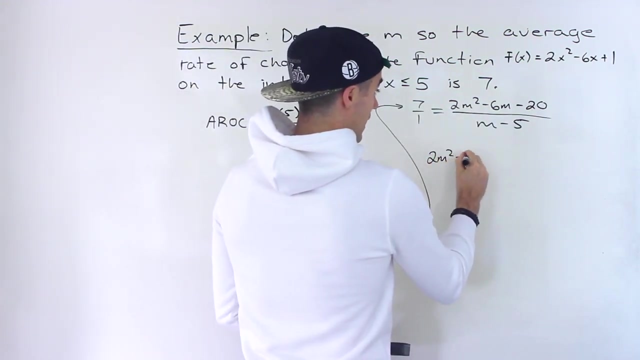 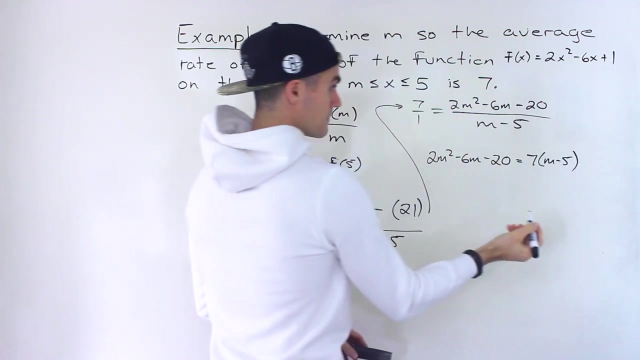 minus 6m. 1 minus 21 gives us minus 20 all over m minus 5, like that. the reason why I put this 7 over 1? because now we could cross, multiply so 1 times. this would just give us that and then we'll have 7 times m minus 5, like that, and then we'll have 2m squared minus 6m minus 20. 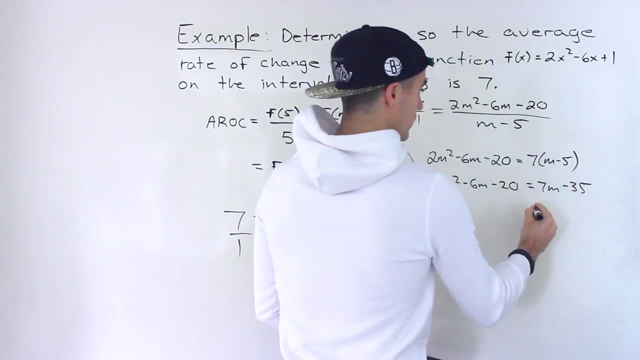 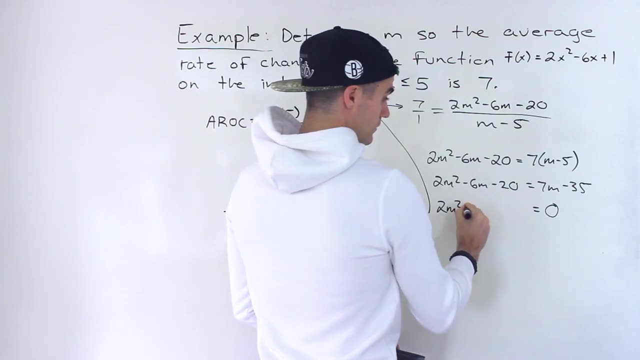 equals 7m minus 35. so when we bring everything over we'll have 2m squared. bring the 7m over minus 6m. minus 7m gives us minus 13m, and then negative 35 becomes positive, 35, negative 20. 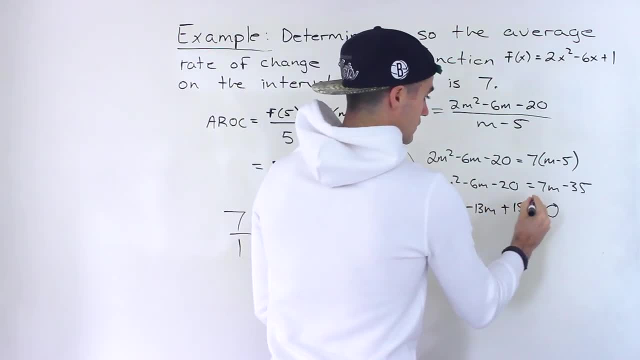 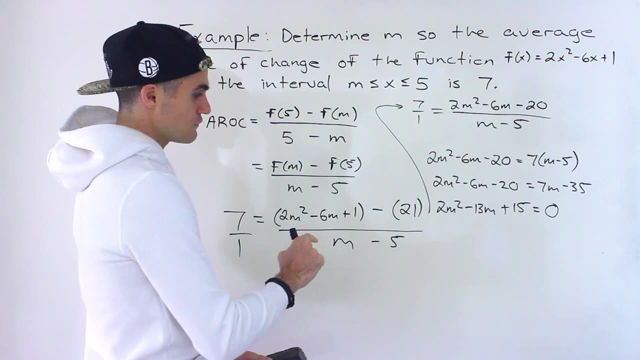 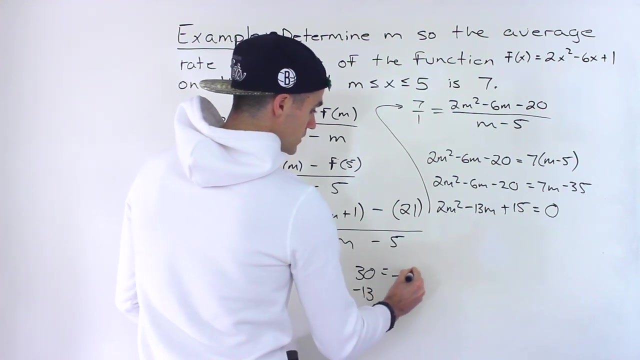 plus 35 gives us 15.. so now we just have a quadratic equation to solve, and this actually factors smoothly because, notice, 2 times 15 gives us 30, and then the b value is negative 13. so what? two values multiply to 30. 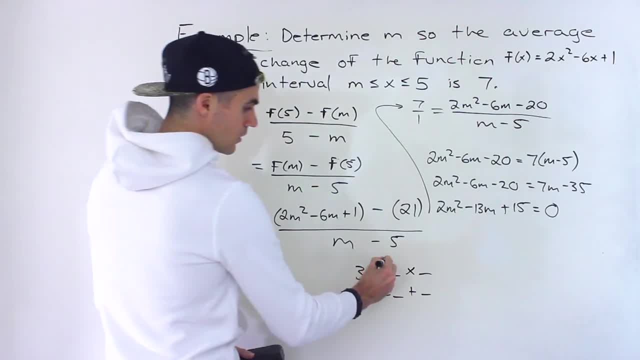 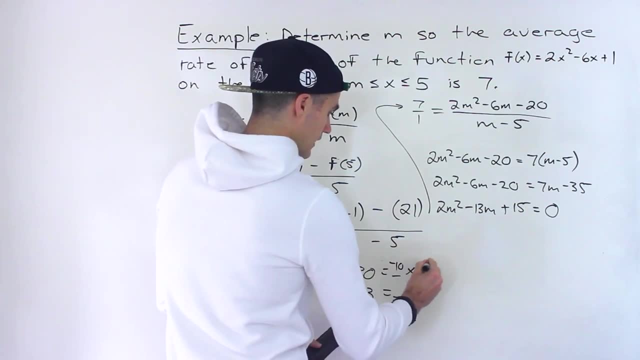 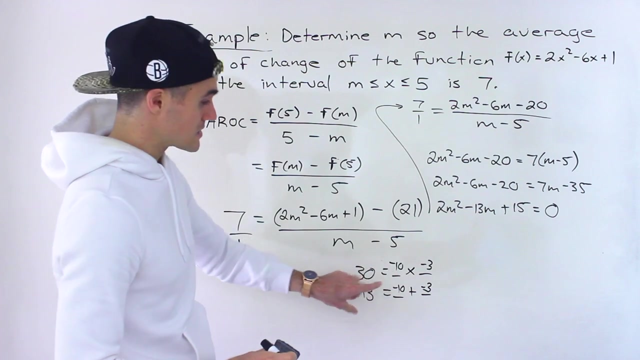 and add up to negative 13. well, it would be negative. it'd be negative 10 and negative 3. right, because we're going to have a quadratic equation to solve. so now we just have a quadratic. is be careful here, because I almost just made this mistake, because 15 and 2, 15 times 2, gives us 30. 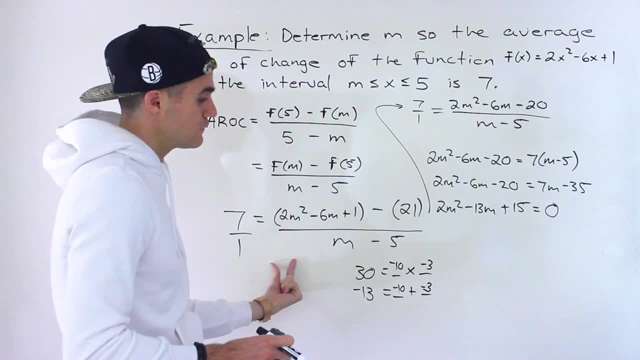 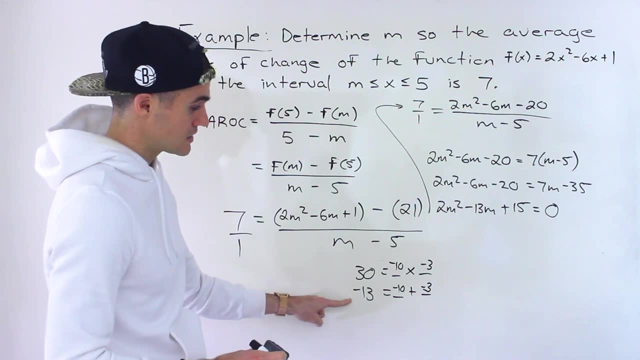 but 15 plus 2 would give us 17. or if we did negative 15 times negative 2, that would give us 30, but then negative 15 plus negative 2 would give us negative 17.. so the two values are negative 10. 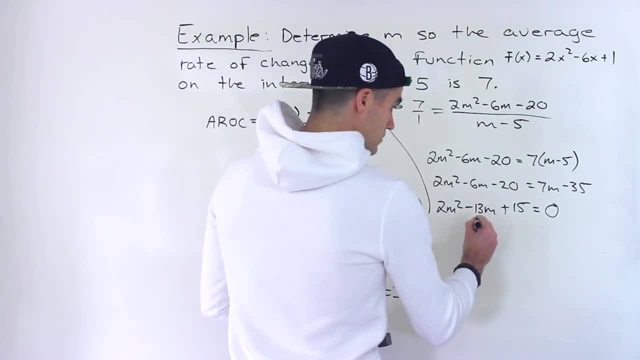 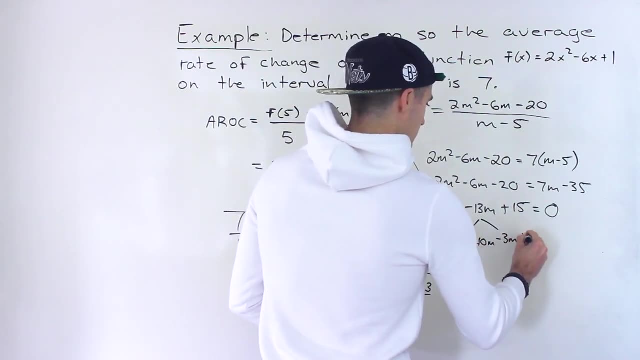 and negative 3.. so what we can do is decompose this to those two numbers. like that notice, we could take out a 2m m minus 5, minus 3 m minus 5, and then we could factor out the m minus 5 and we're left with 2m minus. 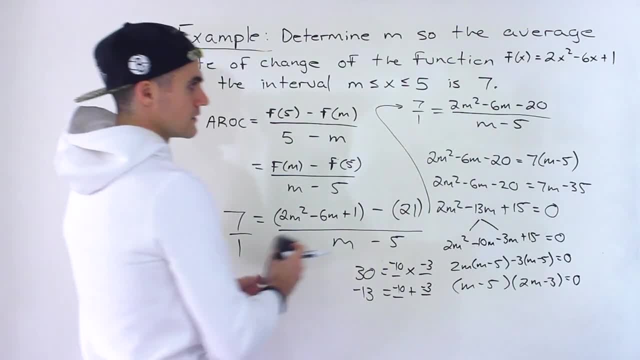 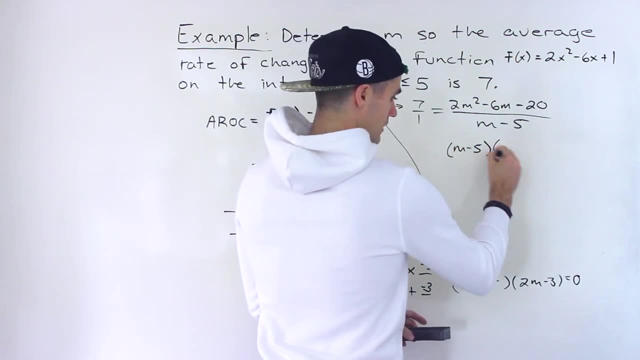 3 like that. so ultimately we end up having: m minus 5 is times. 2m minus 3 is equal to 0, and so from here, m minus 5 is equal to 0, or 2m minus 3 is equal to 0. 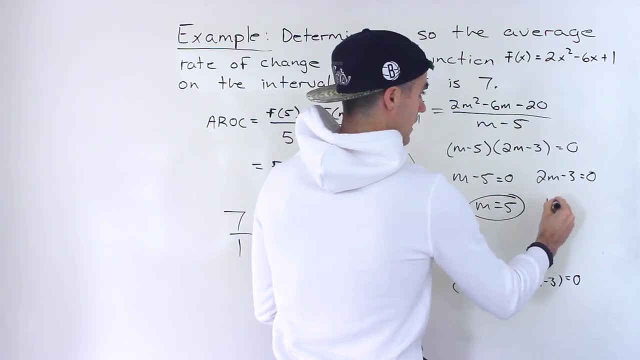 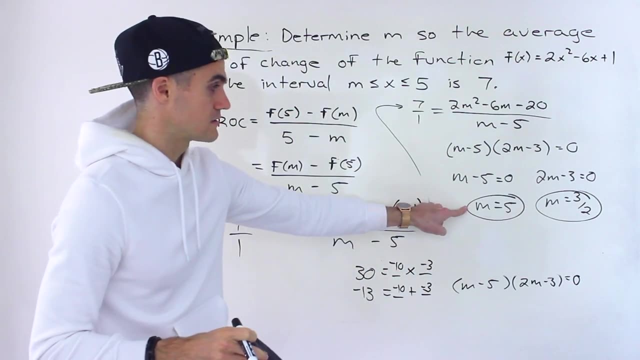 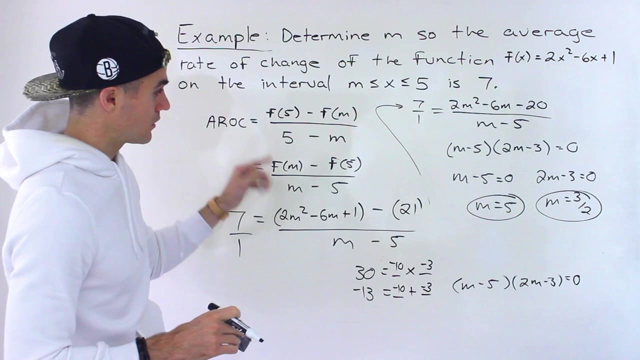 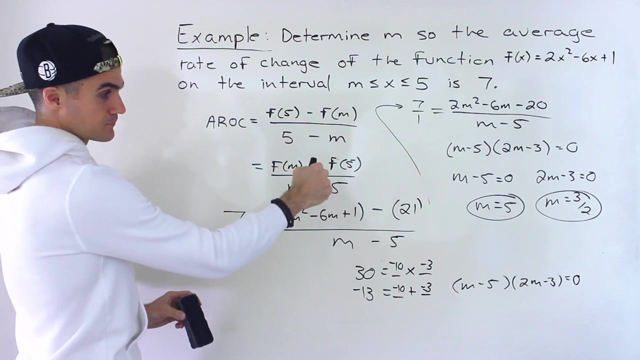 notice here m would be 5. then notice here m would be 3 over 2. now notice that in this particular question this is not going to work. why? because you can't have a zero in a denominator. it would make it undefined, right. so over here, m um equaling five. that's actually a restriction. m can't be five. 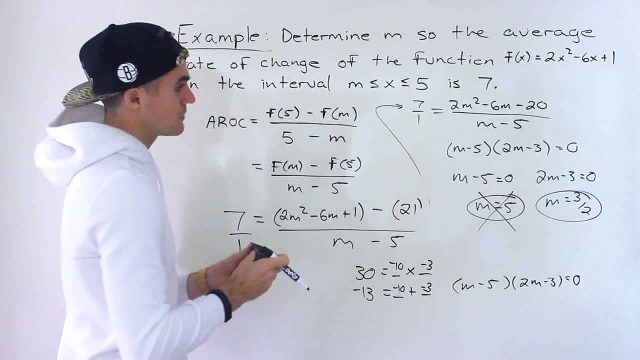 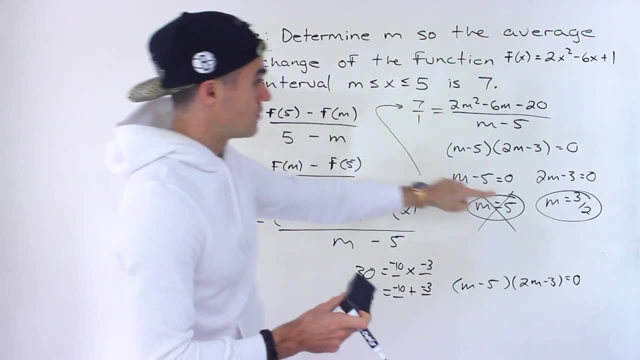 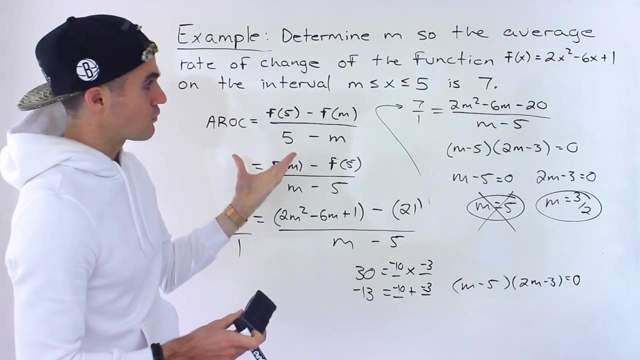 so we would actually just ignore this solution also wouldn't make sense. taking the average rate of change from five to five, right? so this here ends up being the solution: three over two, right? so m is equal to three over two. and then, if you want, if you have the time, you could check it. so